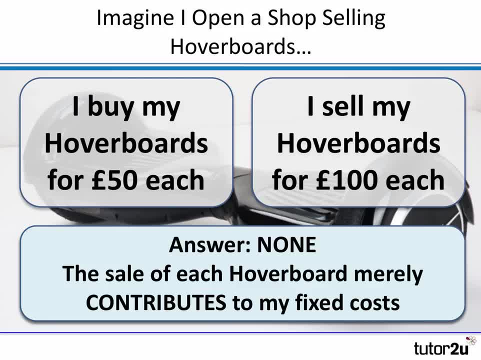 £50, that's not right. The answer is: I don't make any profit at all on buying for £50 and selling for £100. I merely contribute. the sale of each hoverboard merely contributes to my fixed costs. because I've opened a shop, I'll have fixed costs trying to sell these things. So the concept: 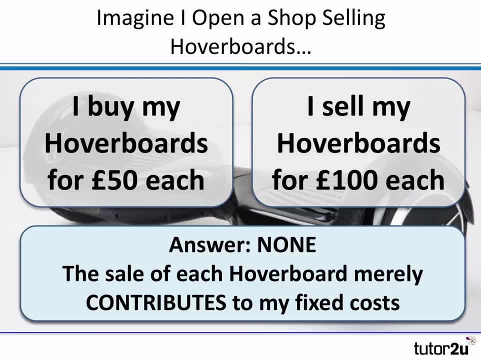 of contribution is this idea that by selling items I can create some kind of contribution to my fixed And once those fixed costs are covered are matched thereafter each time I sell one of my units. it will contribute directly to profit. And that's the idea of contribution. 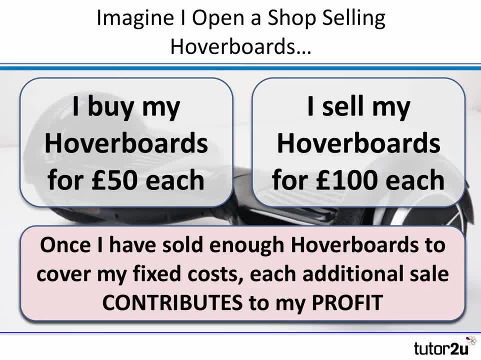 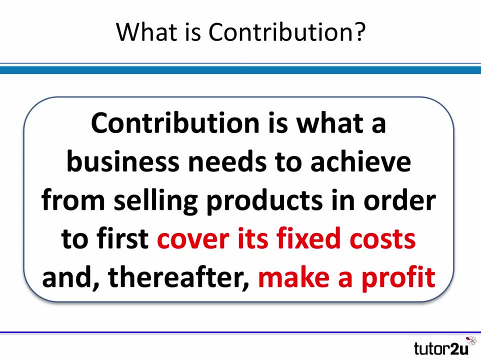 Once I've sold enough hoverboards to cover my fixed costs in the shop- perhaps my rent and my rates and my insurance, maybe having somebody working in the shop to take the orders Once I've sold enough. my additional sales contribute directly to profit, So contribution therefore. 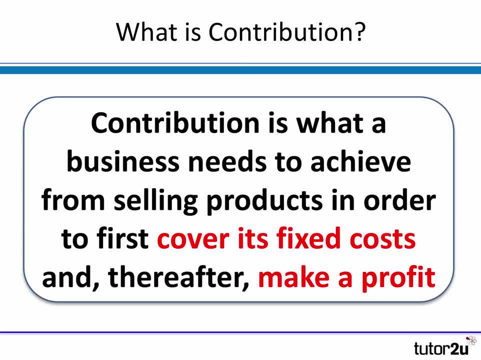 a really important concept is what the business needs to achieve in order, first of all, to cover its fixed costs and thereafter make a profit- A really important concept. Let's have a look at contribution in a little bit more detail to illustrate how it's calculated. 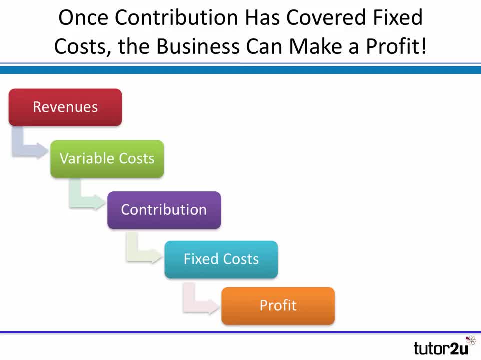 Now the important point is that once I've covered my fixed costs with my contribution, every additional unit should go straight through to profit. Let's just illustrate that with this simple example. In this case, I've got revenues of £100,000 in my business, My variable costs. 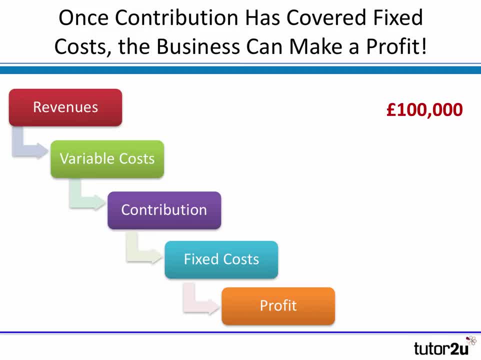 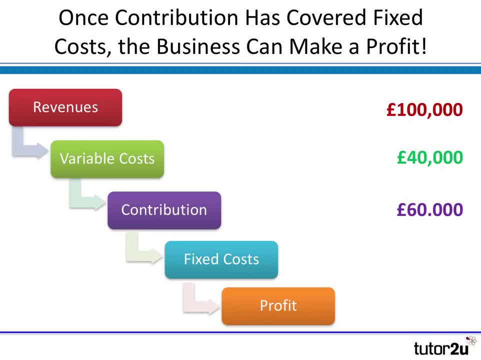 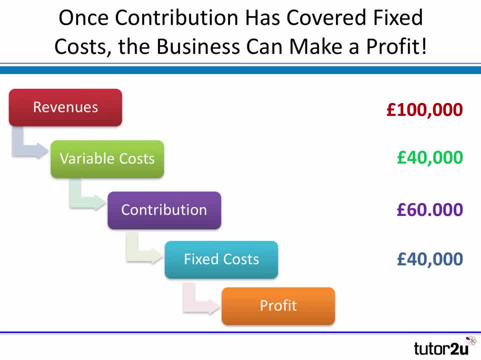 Let's take a look. The fixed costs in this situation are £40,000.. So I've covered my £40,000 worth of fixed costs with my contribution of 60. That should leave something left. It's called profit. Profit is the difference between contribution less fixed costs. So in that case, 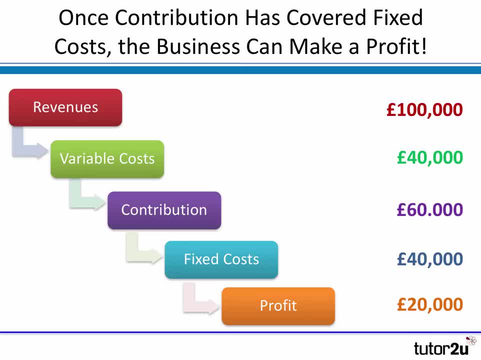 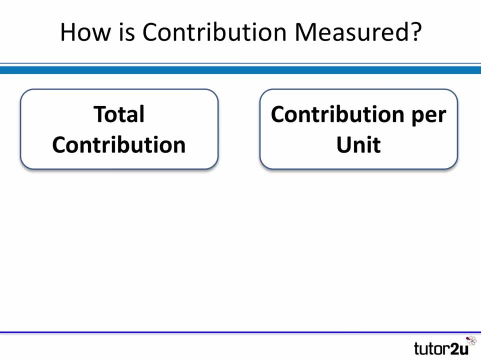 my contribution was more than enough to cover my fixed costs. I'm operating at a profit. There's my contribution: £60,000.. Now how do we measure contribution? There are two important measures that you need to be familiar with and need to practice, And in particular, the one on 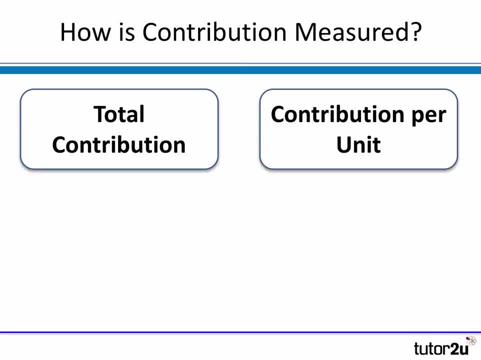 the right contribution per unit is incredibly useful if you're asked to calculate what the break-even level is or the break-even output. Total contribution is calculated by taking total revenues for the business and taking away the total variable costs to the business. So in any 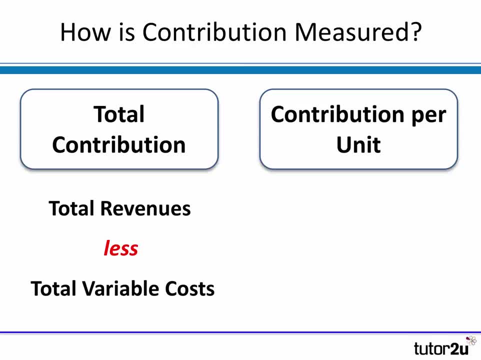 business, you're going to have to calculate the total variable costs to the business. So in any business you're going to have to calculate the total variable costs to the business. So in any business you can usually split costs into those which are variable and those which are fixed For. 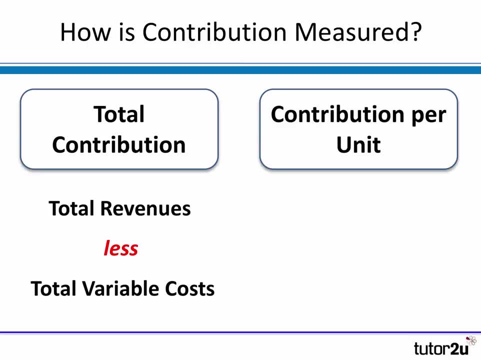 contribution. we are only interested in variable costs. It's total revenues less total variable costs. Contribution per unit is similar, but what it does is it takes account of how many units we're selling. So we take the selling price per unit and we take away the variable cost per unit to give us. 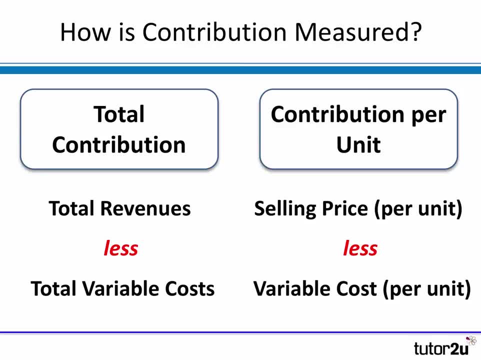 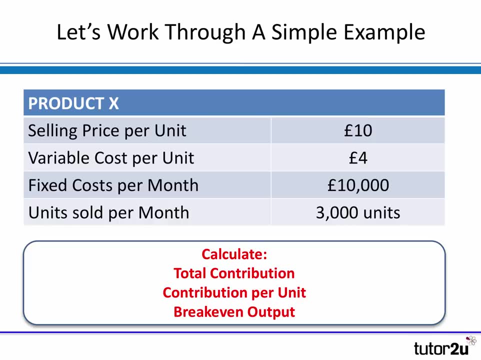 contribution per unit. That's a really important formula to remember, as is the next one that's coming up in a slide or two. Contribution per unit is an incredibly useful concept. Now let's just work through a simple example of how this feeds through in terms of working the maths on contribution. So here we go. There's an example. 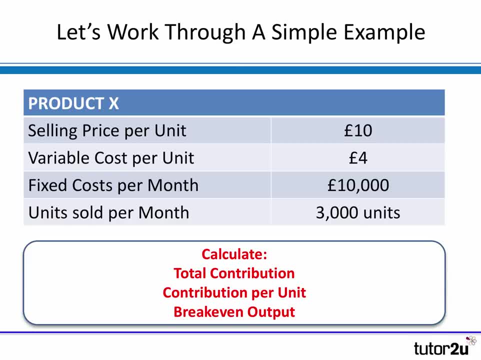 on the screen there. Product X has a selling price per unit of £10 and a variable cost per unit of £4. So here's an example of a selling price per unit of £10 and a variable cost per unit of £4.. We're told that the fixed cost of the business each month are £10,000, £10,000 per month. 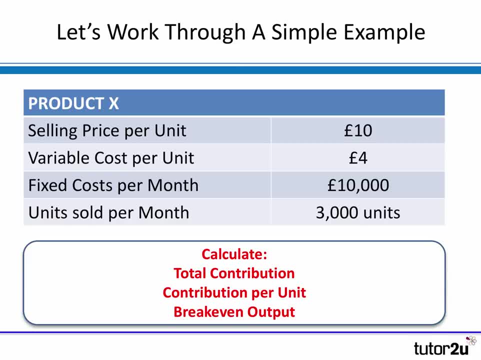 and we're also told that the business sells 3,000 units of product X. Okay, so it's a one product business. We have some selling and variable cost per unit information. We've got some fixed cost information and we're told how many units are sold. So we've got all. 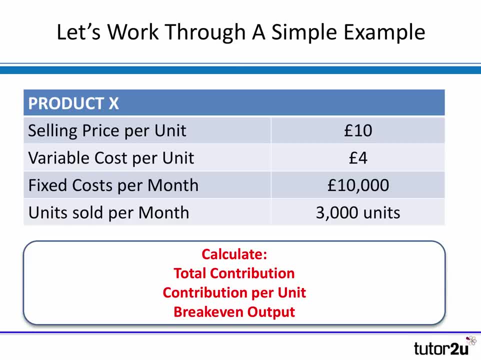 the information we need to calculate total contribution and contribution per unit. But we'll also see that we can use the same information to calculate the break-even out processes. Let's have a look. Well, first of all, let's work out the first two. So the contribution. 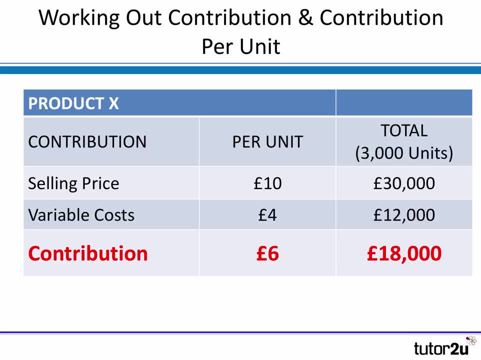 per unit we remember as being the selling price less the variable cost per unit. Selling price was £10.. The variable cost per unit is £4.. Therefore, contribution per unit- £10 less £4- is £6 per unit. Every time I sell one of these units of product X, it contributes £6.. So I've got a. 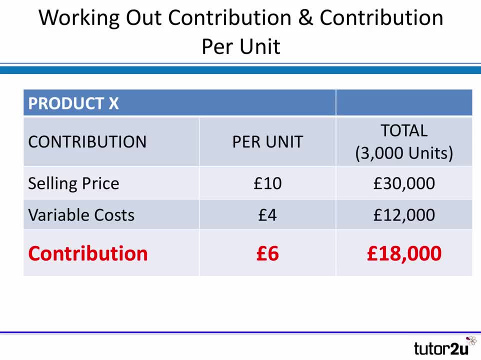 total contribution of £6 towards my fixed costs And if we calculate the total contribution in that month based on the 3,000 units of product X that we sold, we can quickly see what the total contribution was. We simply multiply 3,000 units by the selling price to find out that our revenues 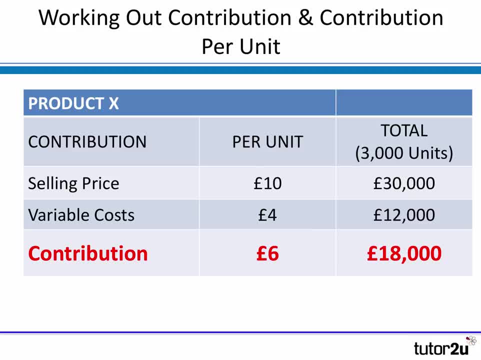 were £30,000 in the month. We multiply the 3,000 units by the variable cost per unit of £4 to work out that our variable costs totaled £3,000.. So we can quickly see what our total contribution was- by 5,000 units of product X. So we can quickly see what the total contribution was. We simply multiply. 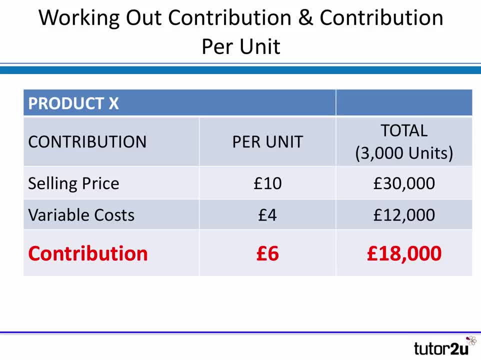 total variable costs were £12,000 and we know that total contribution is total revenues: £30,000 less total variable costs- £12,000. that gives me a contribution towards my fixed costs in the month of £18,000 and of course you can see that £18,000 is the contribution per unit of six times by the. 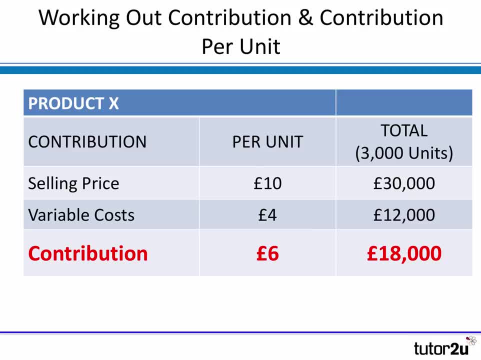 number of units: £3,000. so £18,000 of contribution. now the question is: do we make a profit at £18,000? well, of course, the answer is yes we do, because we want contribution to first of all cover our fixed costs, and everything thereafter is a profit. our fixed costs, I think we were told were £10,000. 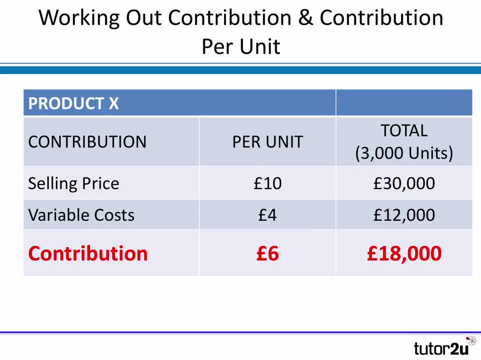 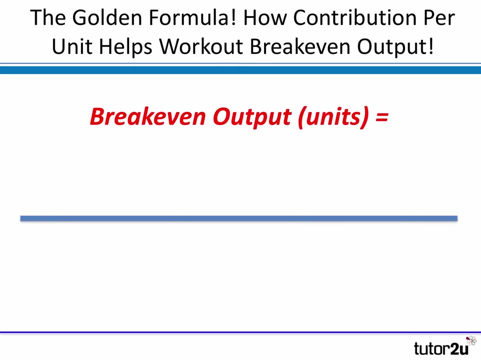 therefore, our profit should be the difference between the two: £18,000 less £10,000. £8,000 should be the profit that we earn in the month by selling 3,000 units at a contribution of £6 each. now, this contribution per unit is an incredibly useful number to work out. 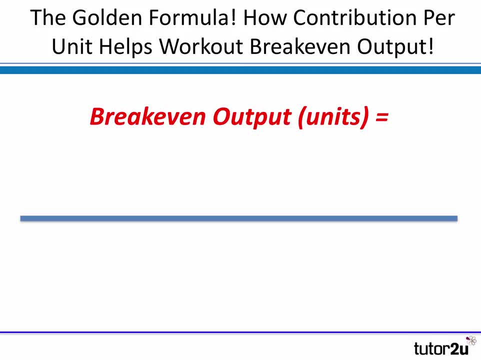 and I'm going to show you how to do that in a moment. and I'm going to show you how to do that in a moment. often you'll be able to get very high marks and use it very effectively to calculate anything to do with the break-even output. don't forget: break-even output is the. 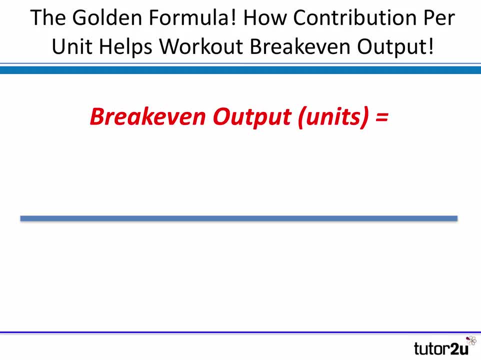 point at which the numbers of units you've made and sold are sufficient to enable revenues to equal total costs. in other words, you're not making a profit, but you're not making a loss. you've broken. you've broken even, and the formula to use is this: break-even output expressed in units. 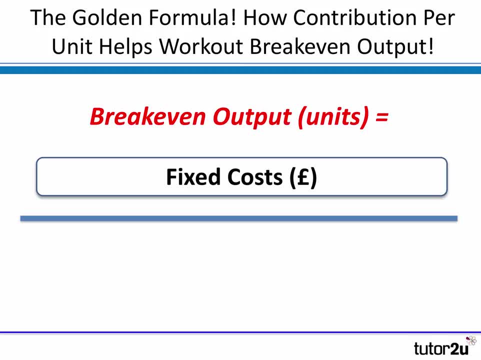 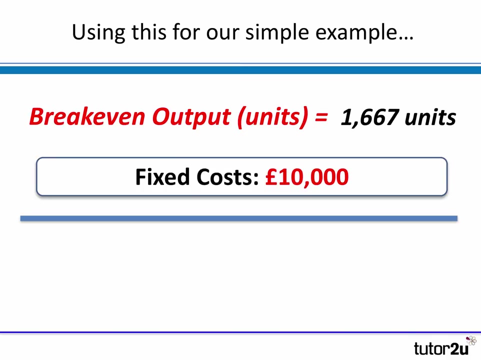 it's calculated as fixed costs: the total fixed costs divided by the contribution per unit. this will always work. so break-even outputs, always expressed in terms of units, is fixed costs divided by contribution per unit. let's have a look using our example. well, I think it's going to be 1667 units. let's check the fixed costs of £10,000. 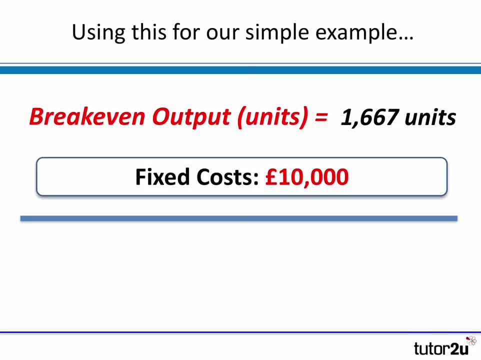 and we know that the contribution per unit was £10 less for £6 per unit. so indeed, £6 per unit is £10 less for £6 per unit. so indeed, £6 per unit is £10 less for £6 per unit. so indeed, £6 per unit is £10 less for £6 per unit. pounds per unit- fixed cost of. 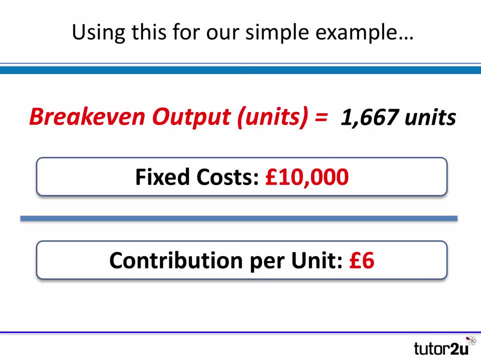 1000 gives you a break-even output of Där­n — 17,000 and 67 units. now we know we're the Arms. per unit fees cost 1000 and gives you an break-even output of第二個 output ofinder 13,000 and. 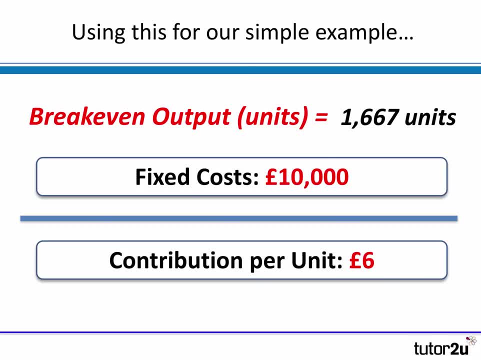 Hours 67 units. now we know we're putting on rent 16,000 units, so no surprise that we are selling more than we need to to break even and therefore we're making a profit in the month. so a quick reminder then. I mean we'll do some further videos. 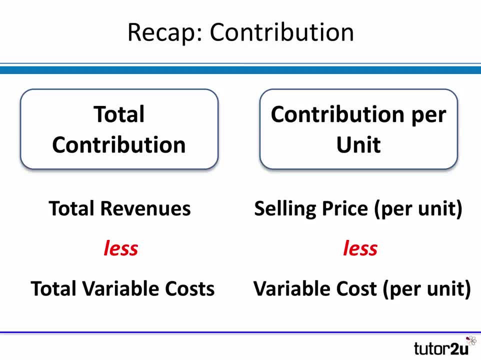 that explained a bit more about contribution per unit and how you can improve a contribution for unit and therefore reduce the breakeven output. so that's a little of what we've covered in other videos. wait until we consider how to convert that right now. so Anve released tonight some of our great numbers from the previous gospos aboutennenachta*.